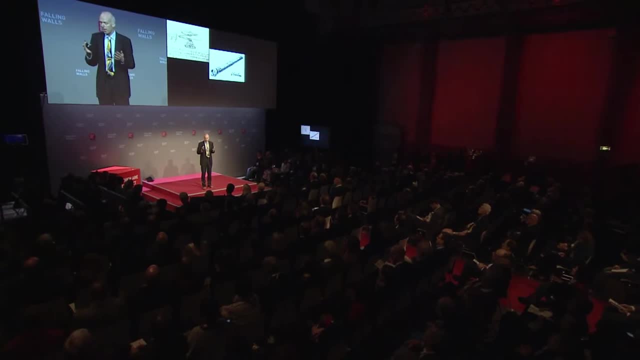 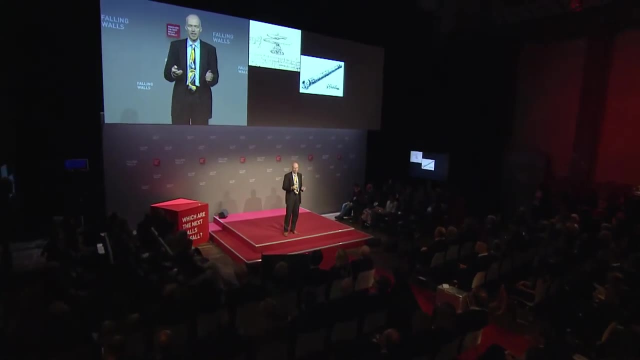 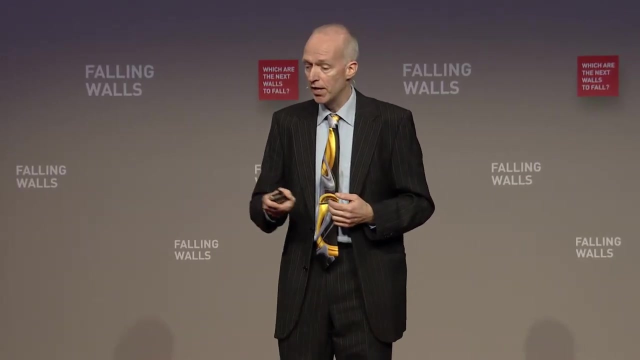 inventions from Leonardo da Vinci and what he invented, And Galileo, how he looked into the moon and to the moons of Jupiter with his telescope, And it was really fascinating for me. I was at a stage that I had to choose enlightenment. I knew what I wanted to do and I knew I wanted to go into science. 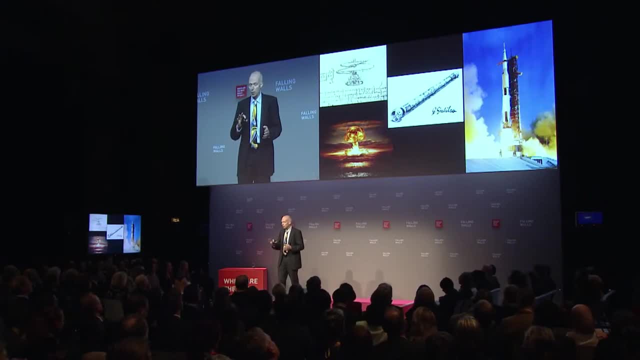 He also talked about space travel and black holes, And he also talked about the nuclear winter. He didn't talk about climate change, but he talked about what a nuclear winter could have for a result that would get a global cooling. When I got into my education with science and with physics, I wanted to do something. 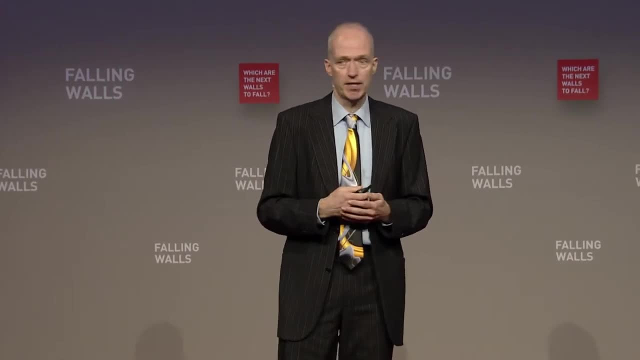 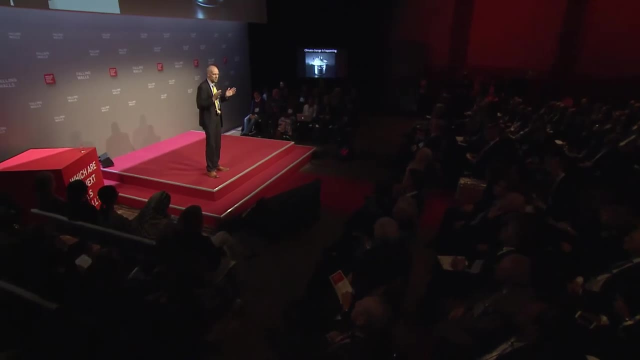 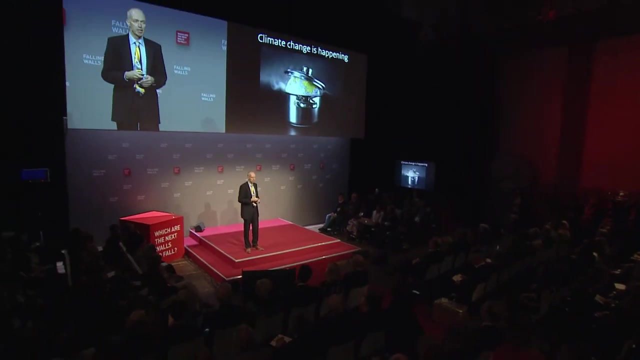 which was relevant for society. So I started to work on ozone layer depletion and climate change, And that's what I'm talking about with you today. Climate change is happening. It's really true. It's happening everywhere. We see the signs not only in the dark and not only far away, but also here in Europe. 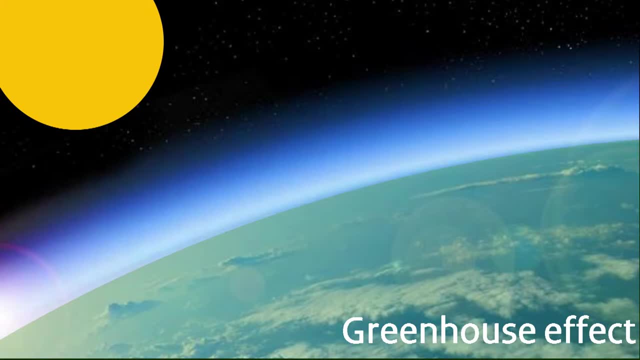 we see the signs And what do we talk about in climate change? A short tutorial. It all starts with the radiation from the sun. The solar radiation hits the surface, hits the earth. part of the radiation is radiated back into space by clouds and just by the atmosphere. And the rest. what comes through the atmosphere warms the surface of the earth, and that's why we have it comfortable here. Part of that infrared radiation is also radiated back into space, and that's good. otherwise it would be way too warm. 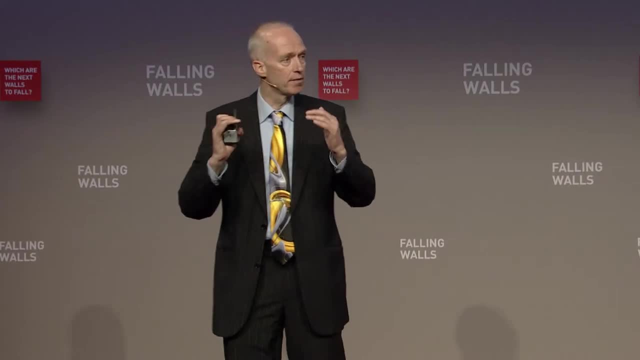 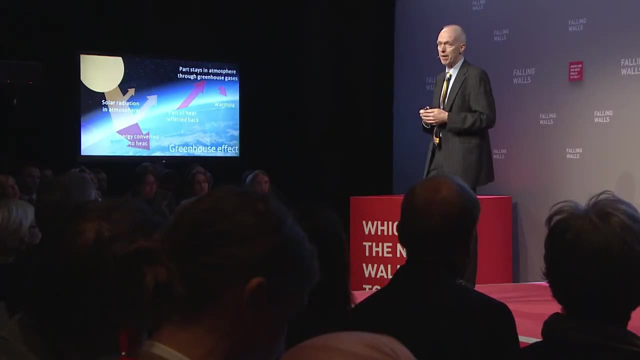 But part of radiation that normally would go out is now hit finds on its way back. it finds molecules, greenhouse gases and therefore extra radiation is put back into the atmosphere. And that's what we talk about with global warming: the greenhouse effect. 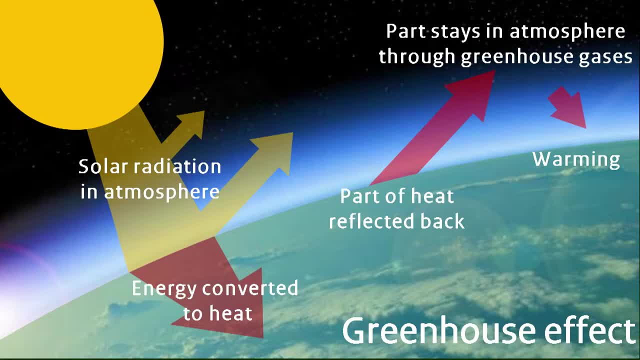 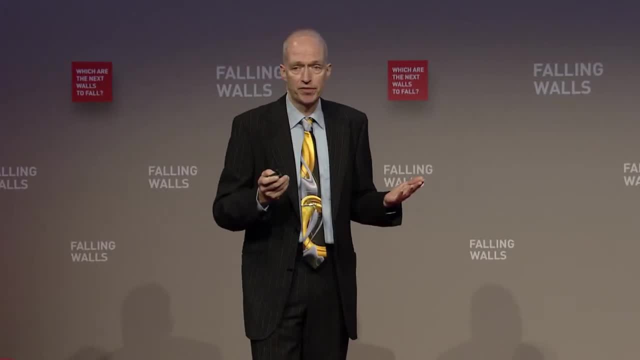 And because we get more and more of these greenhouse gases, more and more radiation is getting back into the atmosphere and that's why it's getting warmer. And as it's getting warmer, the temperature record shows this. These are measurements worldwide, the surface measurements of the earth. 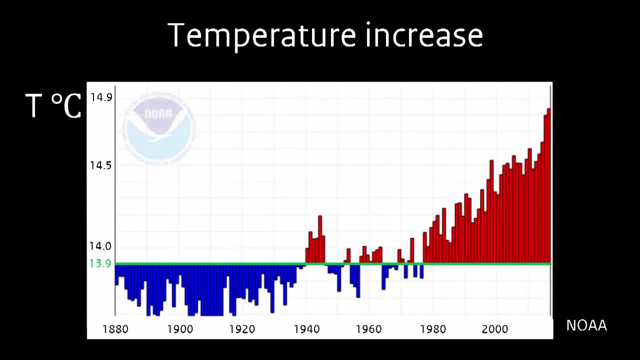 The average temperature over the last century was about 13.9 degrees Celsius And now, since 1980, it has been increasing tremendously and continuously, And we see record after record: 2014 was warmer than every year over the past 100 years. 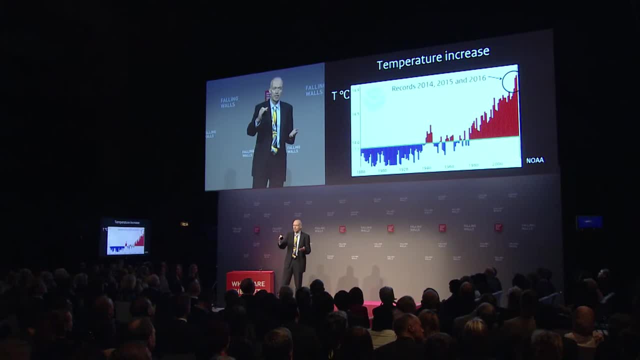 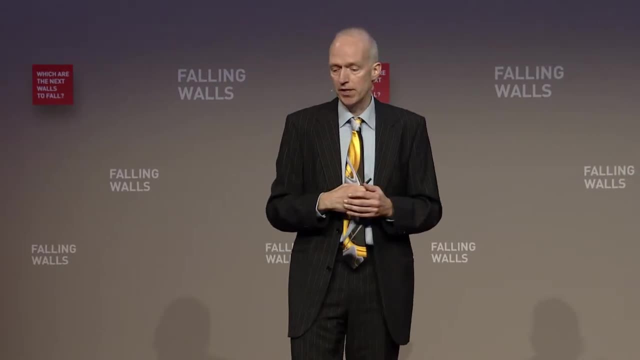 2015 was even warmer again, 2016 was warmer again, And now the projections are that 2014 is even warmer. 2017 will be in the same range as 2015,- 2016.. Clear signals that the world is getting warmer. 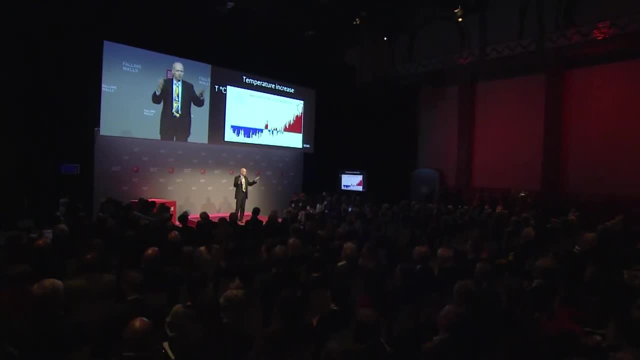 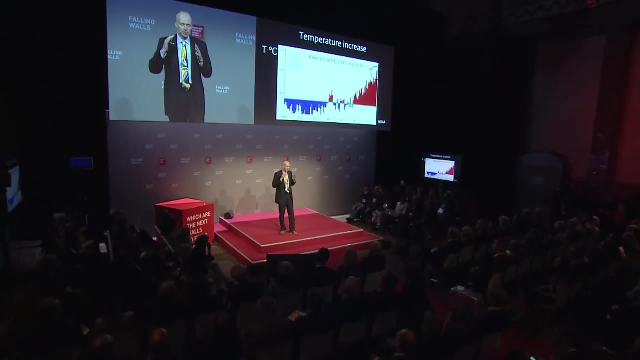 You might say: well, one degree warmer, that's nice here, like a nice summer. But you must remember that one degree here the extremes get also higher, And when you live, for example, in Australia or in Saudi Arabia or in India, and when you 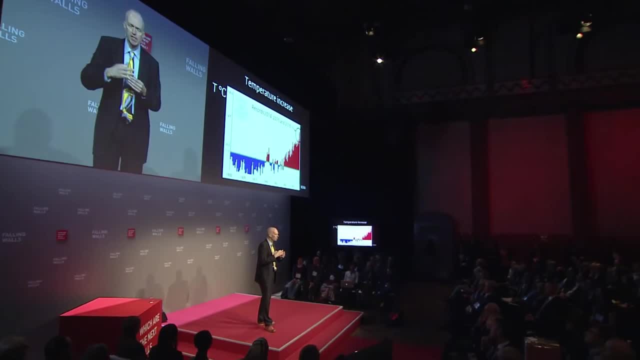 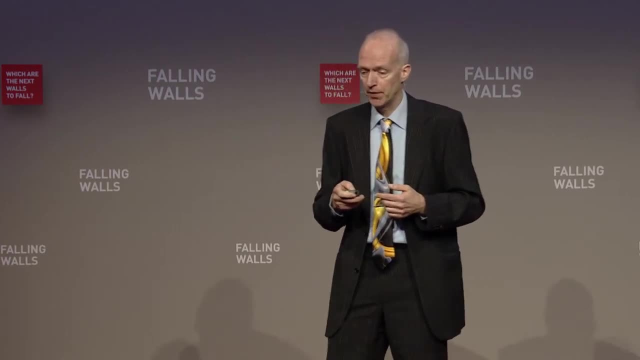 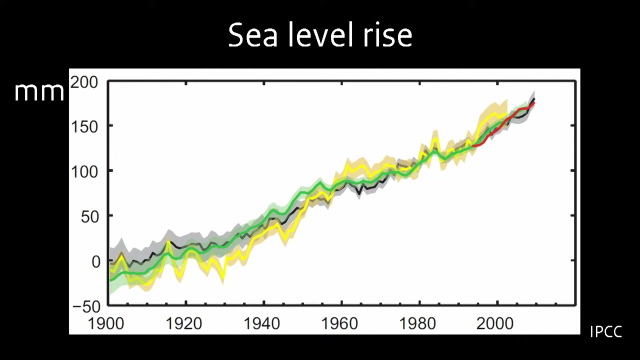 get temperatures like 45, maybe 50 degrees Celsius, then one degree or a few degrees warmer. it's not comfortable anymore. That's really getting a situation which becomes unlivable. Other signs: measurements from the sea level rise. Sea level has been rising about 20 centimeters over the past century and it's projected. 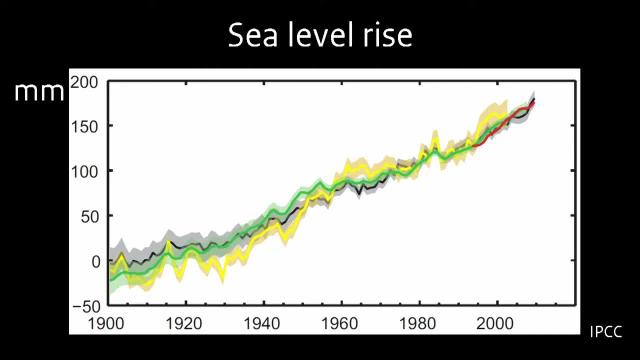 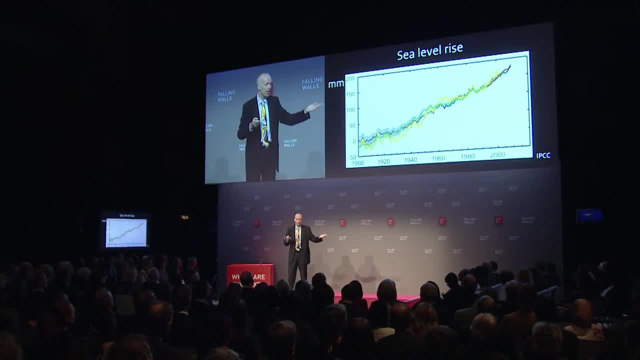 to increase- and it will definitely increase whatever we do- And the increase could be 50 centimeters, maybe up to a meter, And for low-lying states that's a big problem. We live in the Netherlands. There's also sea level rise. 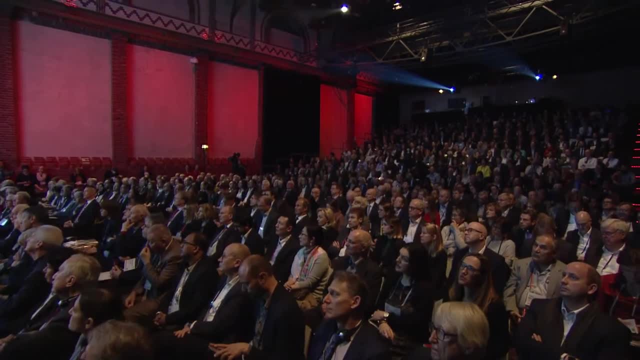 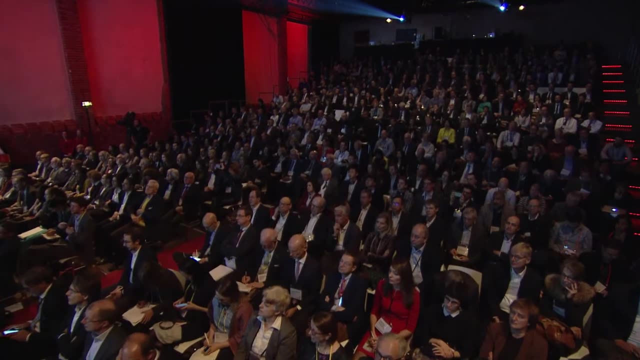 Well, we have the money, We can build a higher dike, We might survive. Then you get pressure off the sea level and then we get the water we cannot use anymore for agriculture. So also in the Netherlands sea level rise is a big issue. 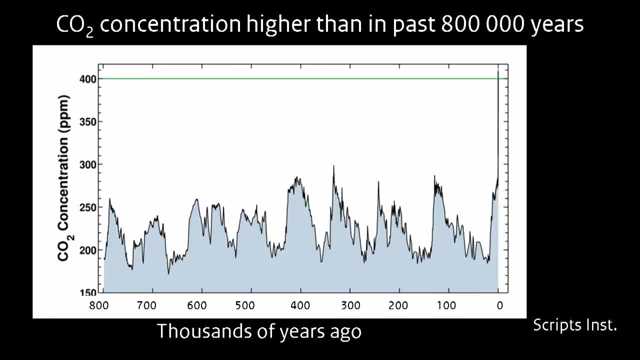 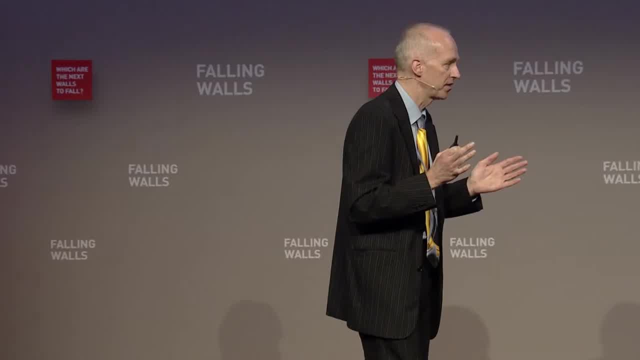 And what's causing this? It's clearly the CO2 emissions- man-made CO2 emissions. Observations show that the concentrations we now have in the atmosphere are higher than they have ever been in the past 800,000 years. These are measurements- measurements in ice cores in the Antarctic. 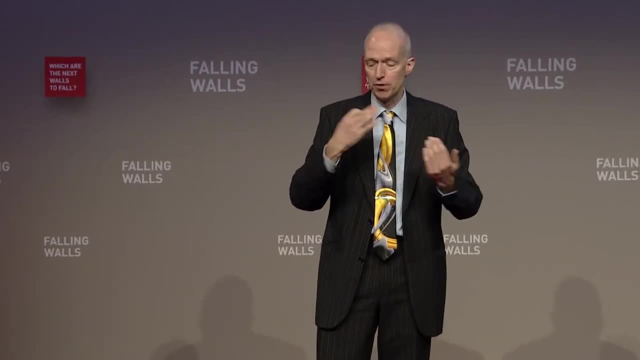 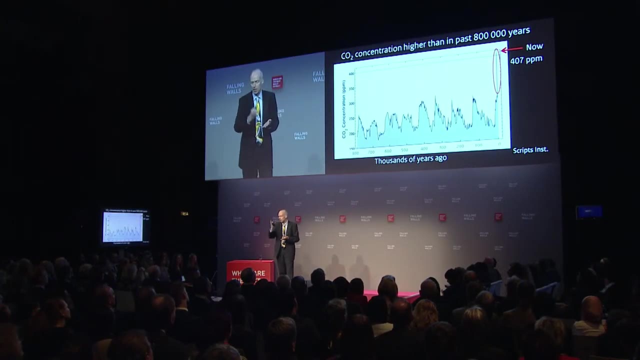 Over the past 800,000 years the concentration was between 200 and 250.. That's a lot- 250 parts per million- And nowadays we have 407.. The last 50 years we've seen a large spike in the increase: 407 now compared to 250 parts. 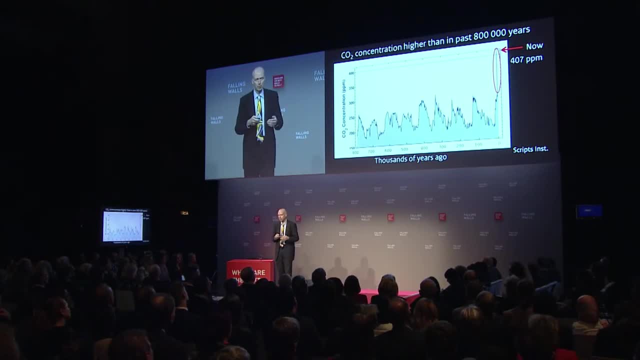 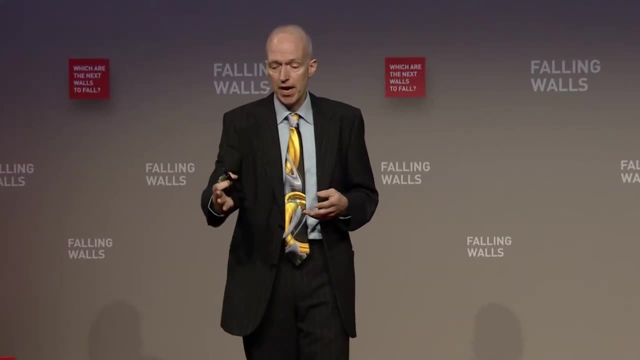 per million over the last 800,000 years- Clearly man-made contribution to climate change. But there are many more effects than just global warming itself. We get droughts. We just had a presentation about refugees, but we can only imagine if the Africa gets. 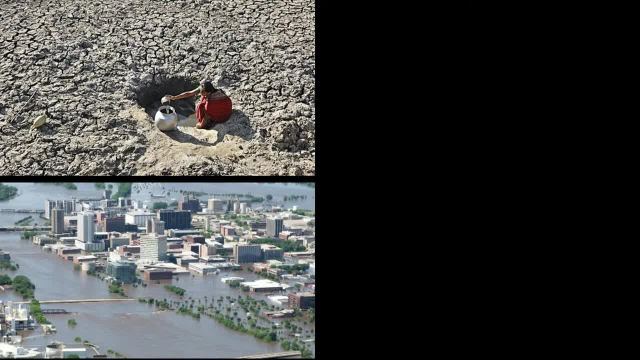 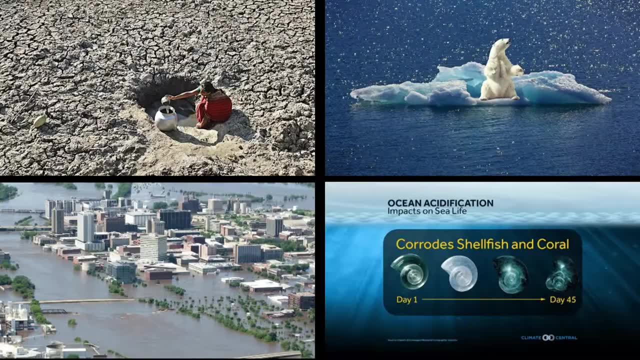 more unlivable? what will happen with the refugee studies? We have flooding, clearly everywhere we sit already now. But also we have the melting of the ice in the Arctic. Probably in the coming decades most of the ice in the Arctic will be gone. 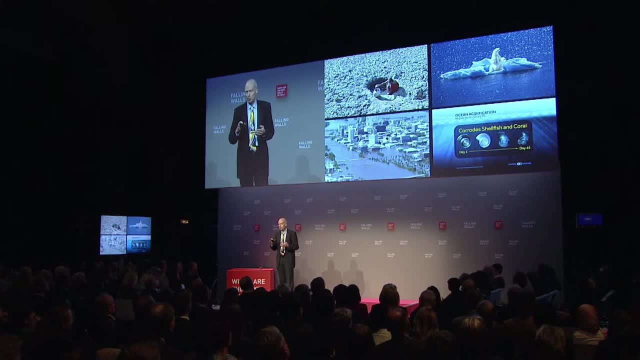 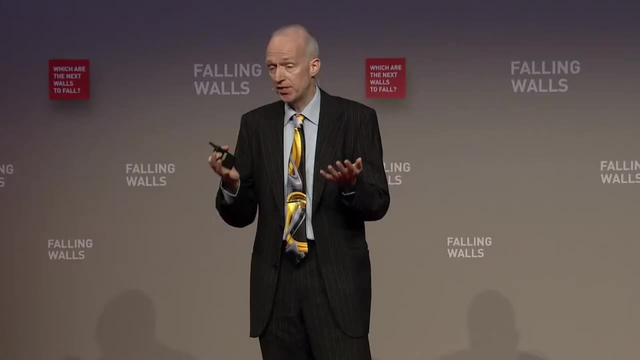 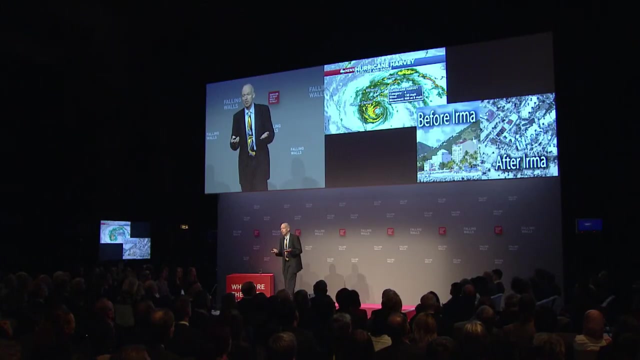 The thing which is underappreciated in the public is that also CO2, carbon dioxide, causes acidification of the oceans and affecting there the corals and affecting there the shellfish. so the beginning of the food chains in the oceans. We've all seen these pictures at the beginning of this year. 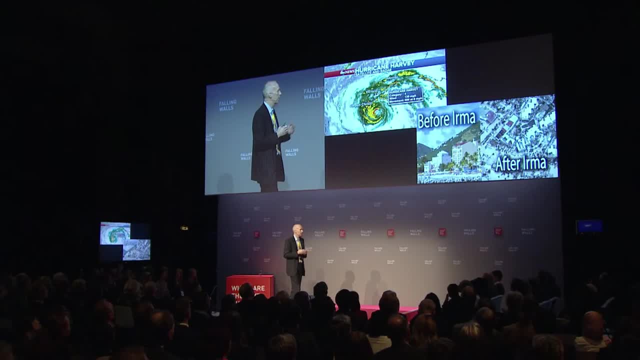 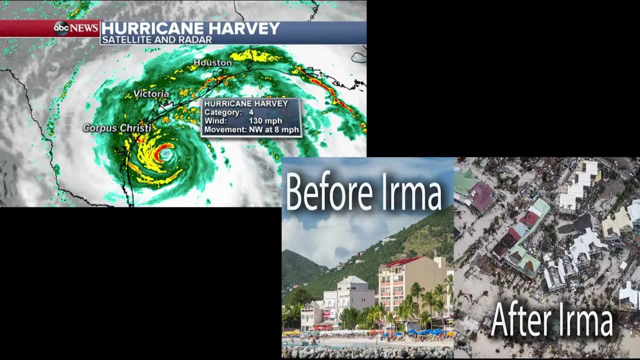 The hurricanes over the Caribbean: Hurricane Irma and the Hurricane Harvey over Texas, Devastating effects from the flooding and the winds. Now, I'm not going to say that this is directly caused by climate change. We don't know A single event you cannot attribute to this. 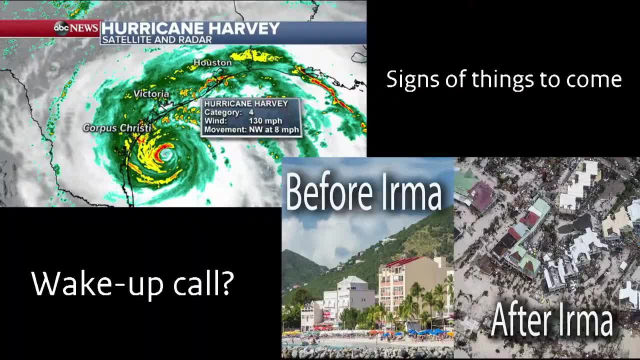 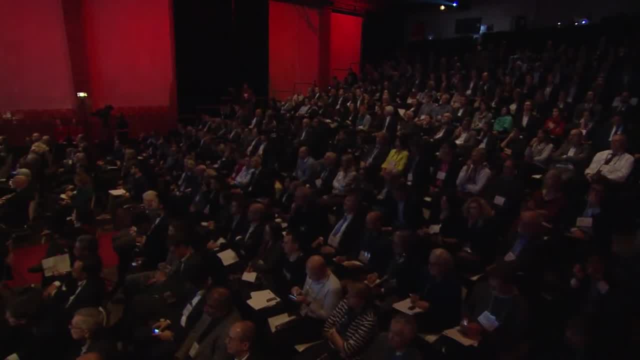 But it's clearly a sign This is something which is likely to happen more. Severe hurricanes are consistent with a warmer climate, So we're expecting these severe hurricanes to happen more in the coming decades. So I think, of course, it's devastating. 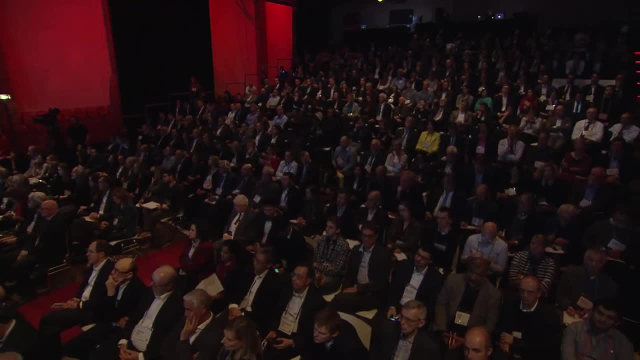 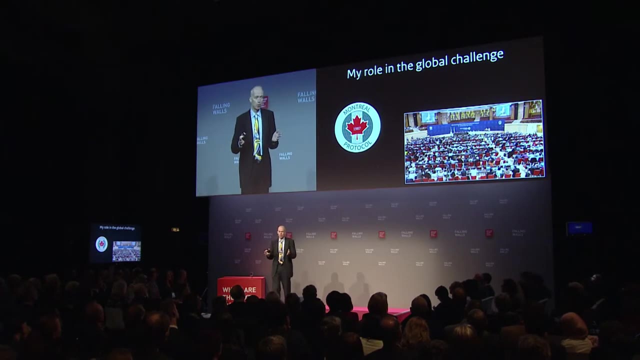 But it might also be a good way to put it. It might be a good way to wake up call for everybody that this is a future we are going to see more. What was my role in this? I've been mostly working on the Montreux Protocol. 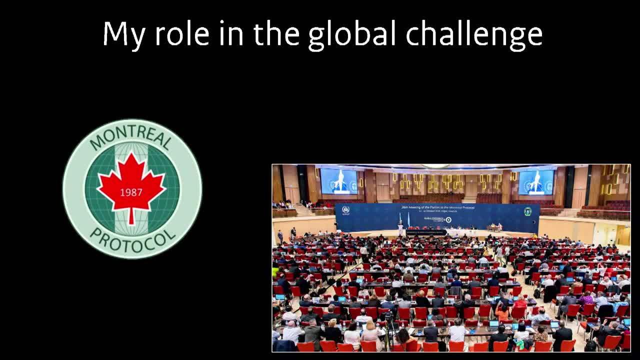 You might remember, the Montreux Protocol is signed in 1987 to protect the ozone layer And I've been visiting these conferences or parties where all the countries are discussing the future of the ozone layer, And I was always sitting there in the back somewhere as a scientist. 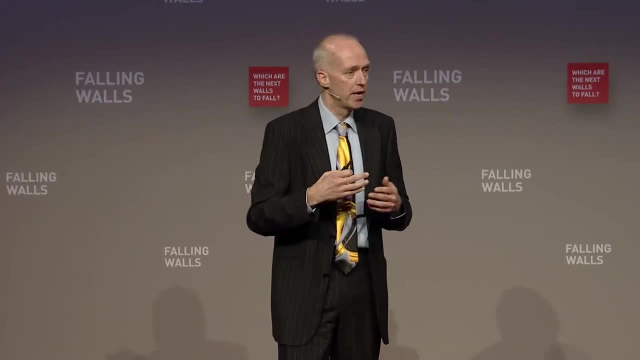 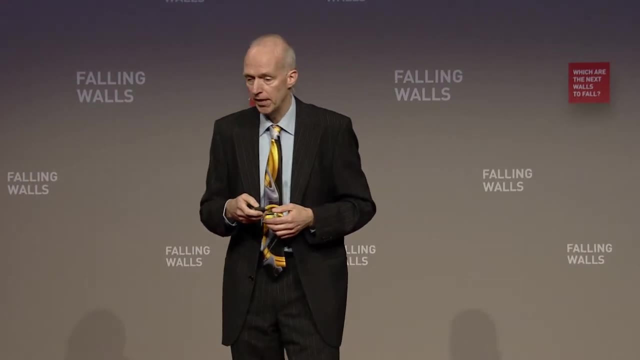 I'm not a negotiator, I'm a scientist And I was always there with my laptop And I did calculations During the discussions to try to convince the policymakers if they were making the right choices. So you think now maybe. why don't I switch to ozone layer depletion? 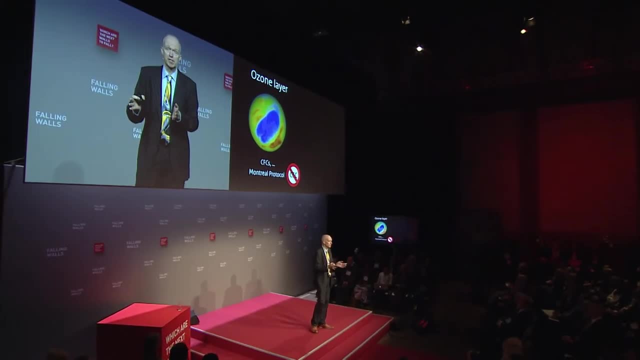 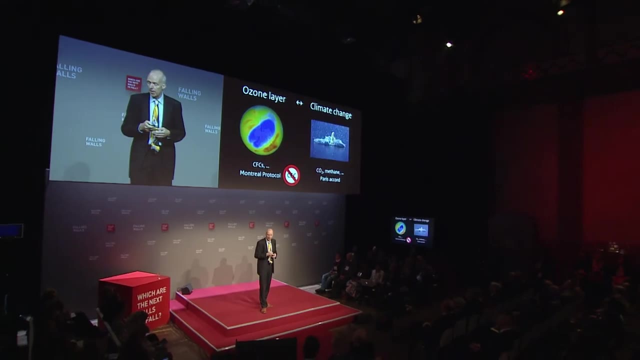 Ozone layer depletion has nothing to do with CO2.. Ozone layer depletion is about CFCs, And the Montreux Protocol has banned CFCs globally. You cannot use them anymore in refrigerators and air conditioners, And there's a different issue in climate change. 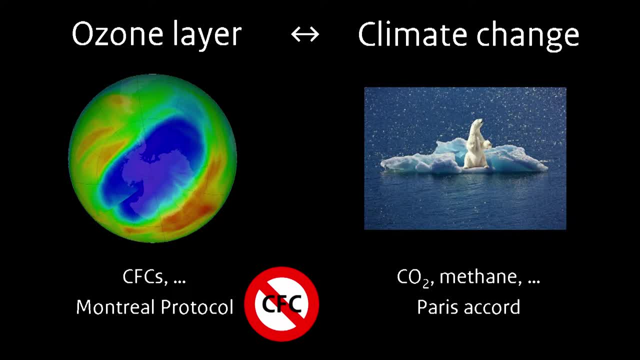 Climate change is about CO2 emissions and methane. And now the Paris Agreement and now the discussions in Berlin with COP23.. How do you counter that? How do you really put a handle on it? So two distinct issues, But they're not so distinct. 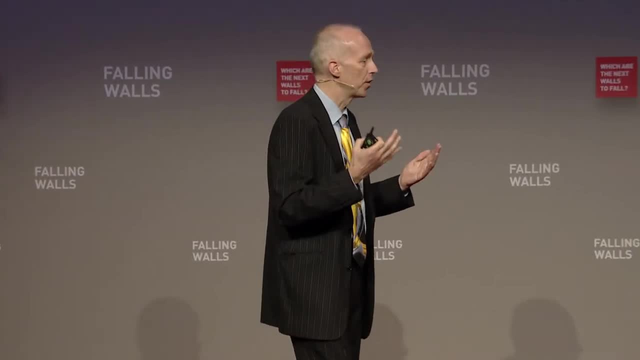 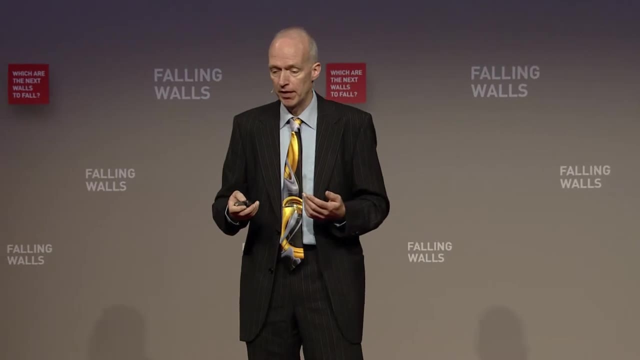 The CFCs. you might remember them by the common name the Freons. They were used since the 1940s, 1950s in air conditioning, in refrigerations, in large amounts And they were discovered by two Americans in 1974 that they could deplete the ozone. 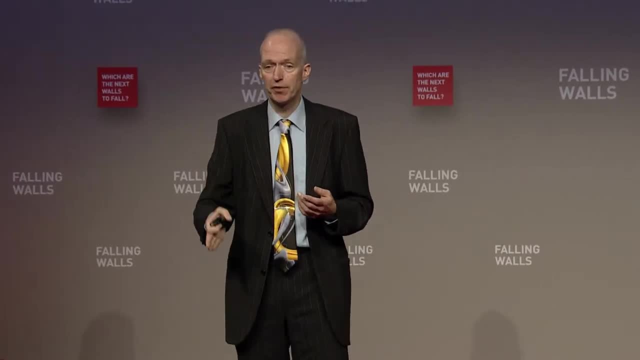 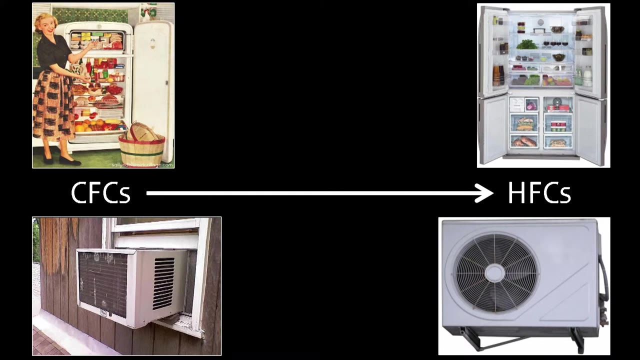 layer. And what happened now? industries switched to different chemicals. They switched to HFCs And now a lot of refrigerators you buy and air conditioners all over the world. That's a big difference. And the HFCs all over the world contain HFCs. It was a very good step for the ozone layer because the HFCs do not deplete the ozone layer, So it was a very good step, But unfortunately, HFCs are strong greenhouse gases, So as a result of one protocol which saves the ozone layer, you didn't find the optimal. 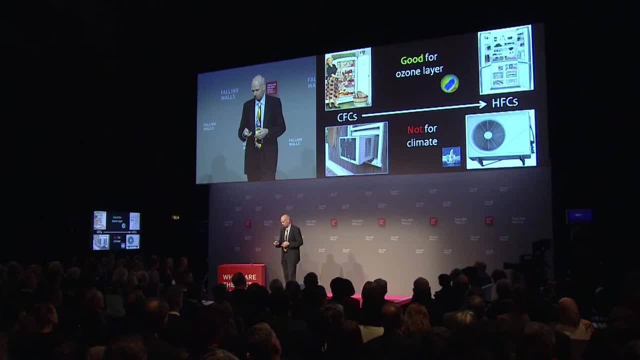 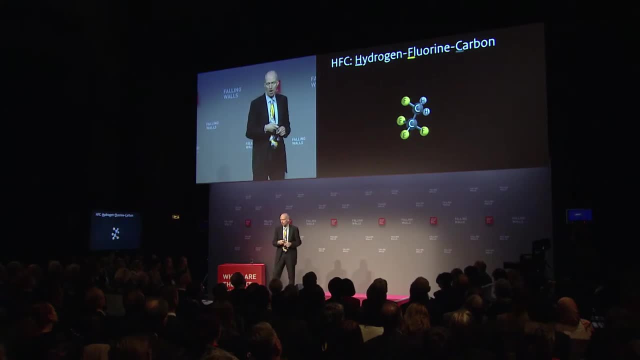 solution, but you found something which creates a greenhouse effect, And that's, of course, an unintended side effect. What are HFCs now? HFCs are hydrofluorocarbons Molecules in the air, Molecules like these, with carbon, fluorine and hydrogen in there. 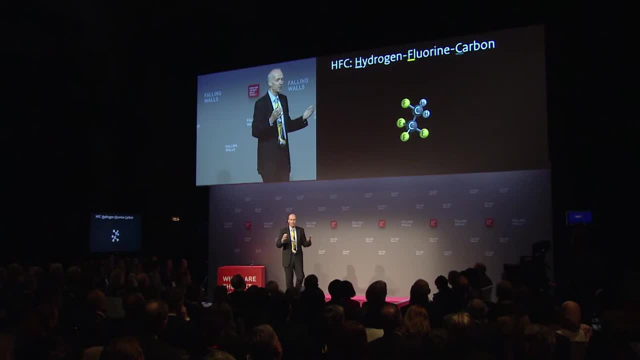 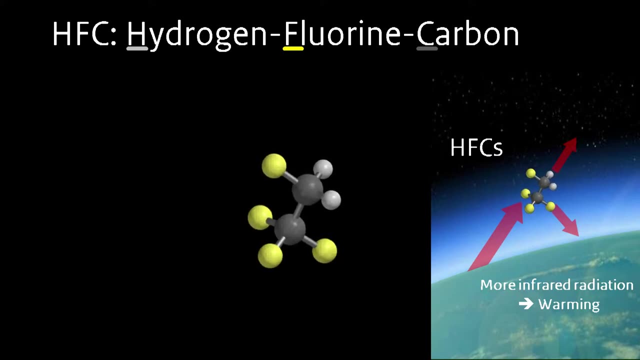 And they have a lifetime in the atmosphere, when they are released, of about 50 years, 50,, 60 years. What's happening when they're in the atmosphere? they start to vibrate. The infrared radiation which is coming from the surface hits the molecules at just the 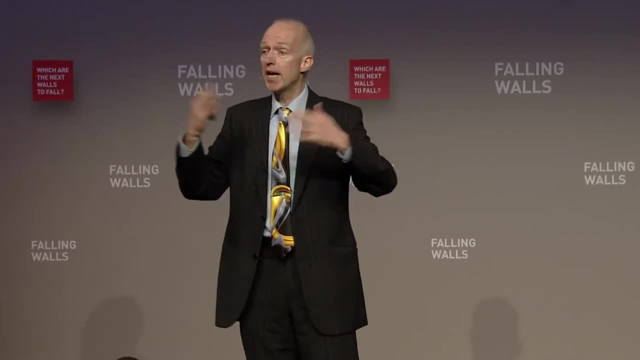 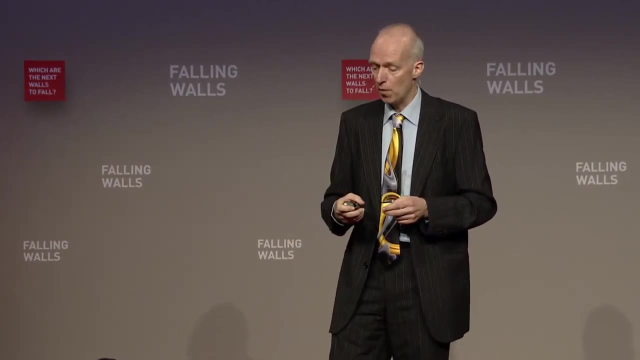 right frequency, They start to vibrate And because they vibrate they radiate infrared radiation back to space, But not only back to space, also back into the atmosphere. So it's causing an additional warming there. And just a few things. 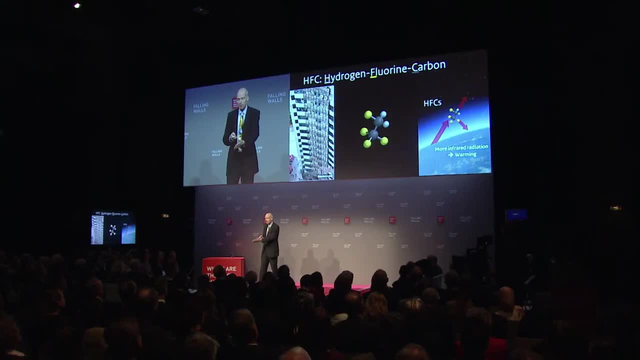 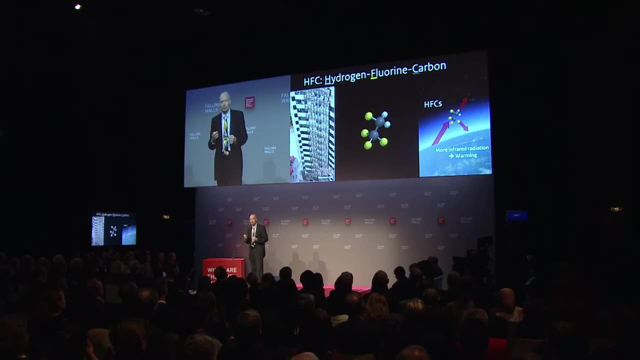 A few molecules wouldn't be such a problem. The projections are that we get these kind of situations, that everywhere we see air conditionings And most of the air conditionings are very leaky. They leak 10, 15% of their HFCs every year. 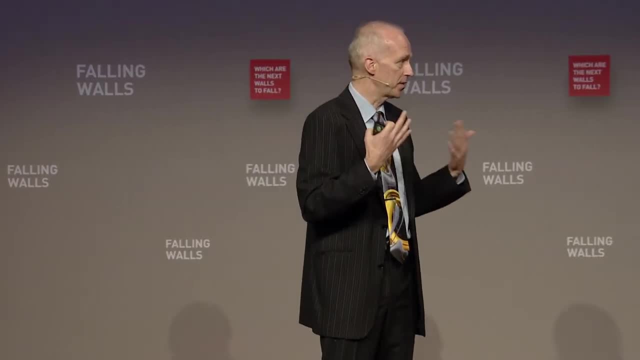 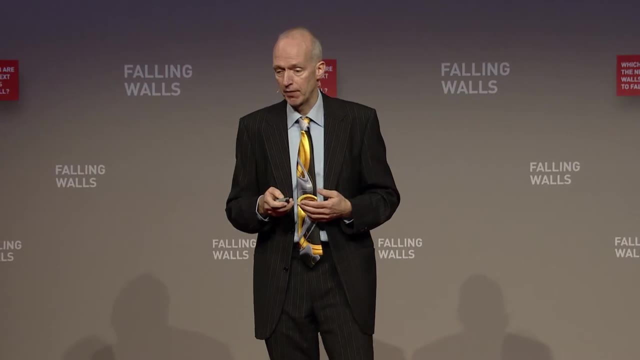 And especially the growth in Europe and in America and in Asia is expected to continue over the coming decades And therefore the HFCs could be a big threat to climate change. What I've been doing in this, I've been doing my scientific work. 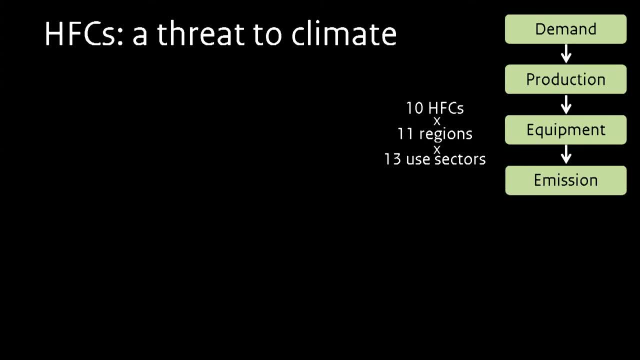 Not only doing the scientific work, I also brought to the policy makers and discussed the results. I've made a model in which I estimated globally what would be the amount of HFCs. Then I calculated the production. How much was in equipment? 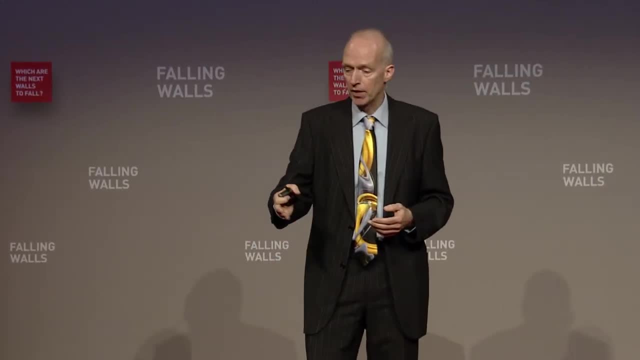 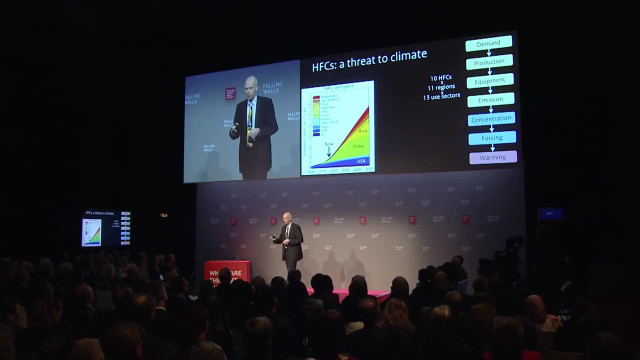 How much are the emissions, Calculate all the way down to global warming. And that I did for all the world regions, all the different sectors that were relevant there, And I produced these kind of graphs which shows you, for the different countries, how much the emissions are of these HFCs over the coming 50 years. 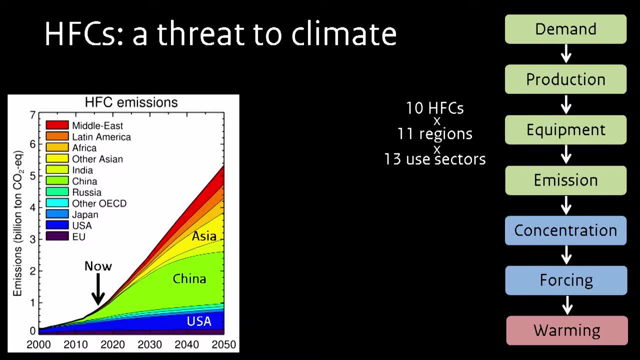 And we see nowadays that it's still the majority Majority coming from Europe and from Asia and from the United States, But the projections are that the majority will come past 2020 from Asia, China, India and other Asian countries. It's now expressed here in emissions in billion tons of CO2 equivalent. 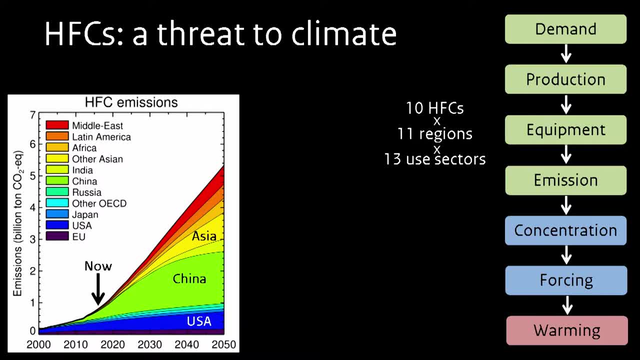 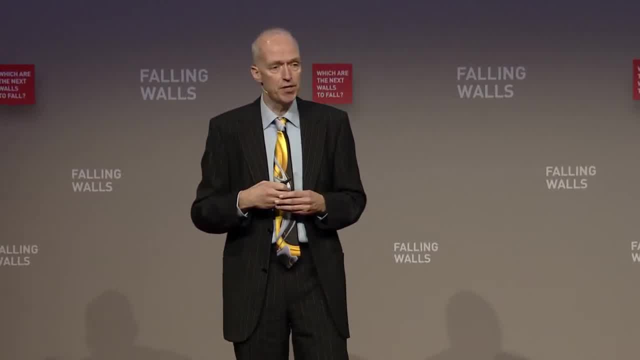 And you might think, wow, that's a number. I have no clue what it is. If you look at the five to six billion ton equivalent, the climate effect of those emissions are the same as the CO2 emissions of 1,500 medium-sized power plants. 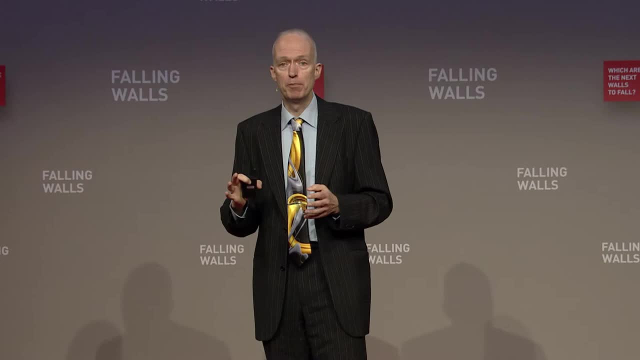 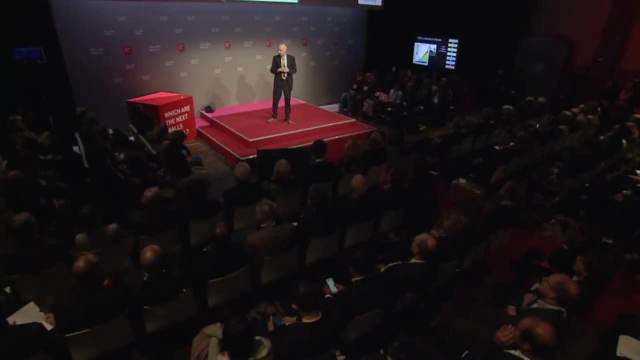 That's a huge amount. Wow. Another way to put it in perspective. for example, you fill this whole room with CO2, with carbon dioxide the main greenhouse gas. The climate effect of that would be the same that if you fill this box with hydrofluorocarbons. 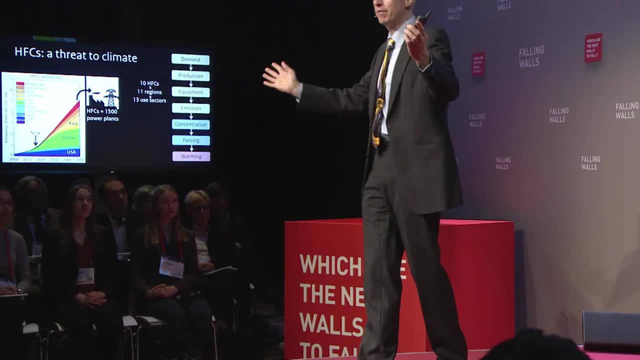 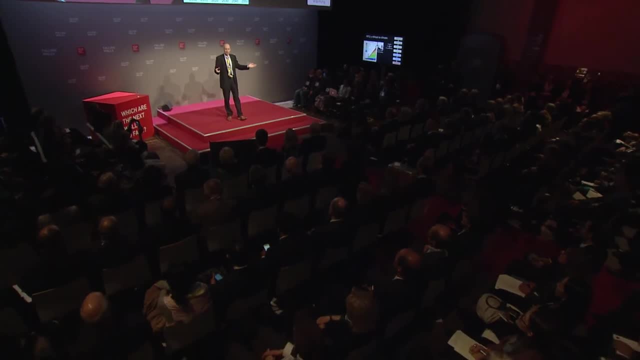 with HFCs. So one small box gives you the same climate effect of this whole room. Another way, what I found very disturbing when I calculated it: when you have this room filled with CO2 emissions- with CO2, fully full- then every year humanity emits three. 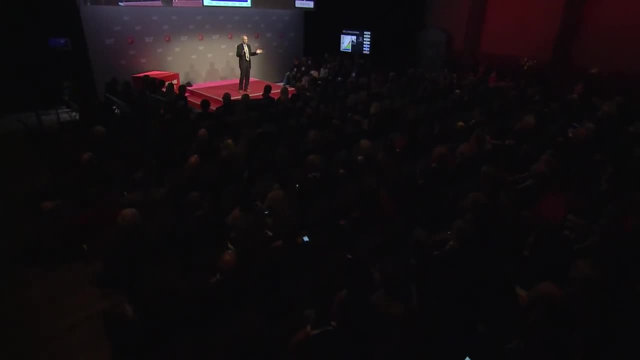 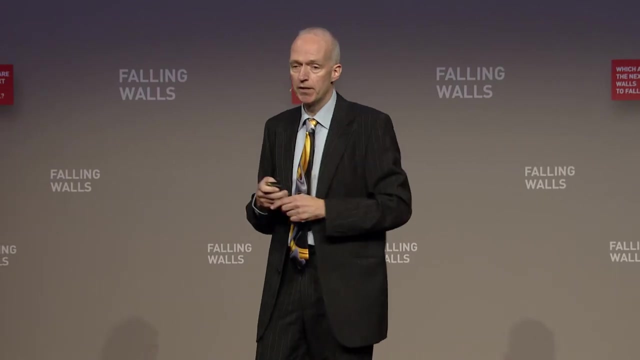 million of these rooms into the atmosphere, Three million rooms filled with CO2.. I find that mind-boggling. How can we do this? What I also did: I communicated with the policymakers. what would this be, in effect, for climate change? 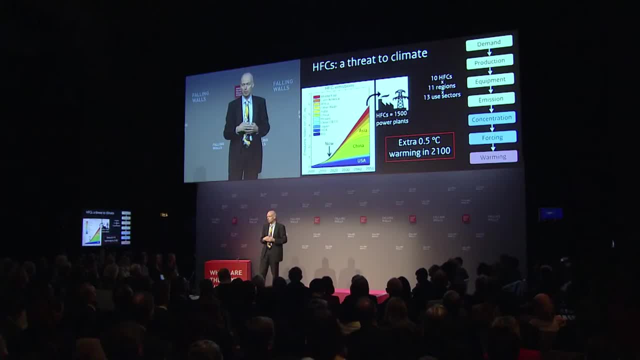 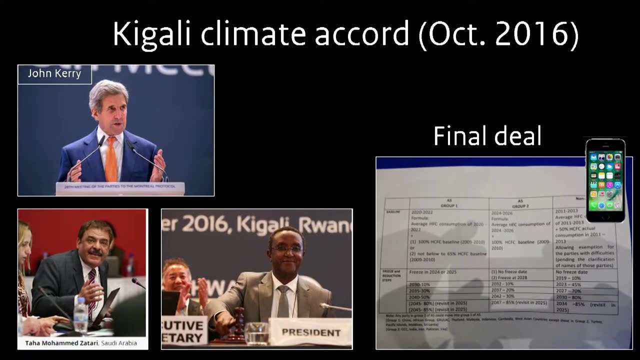 It would be an extra warming of up to 0.5 degrees average surface warming all over the globe, A half a degree warming. and I will put it in perspective. What happened now? last year in Kigali in Rwanda, all the politicians came together after seven. 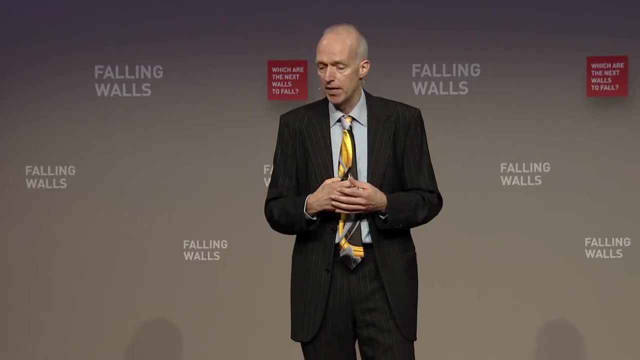 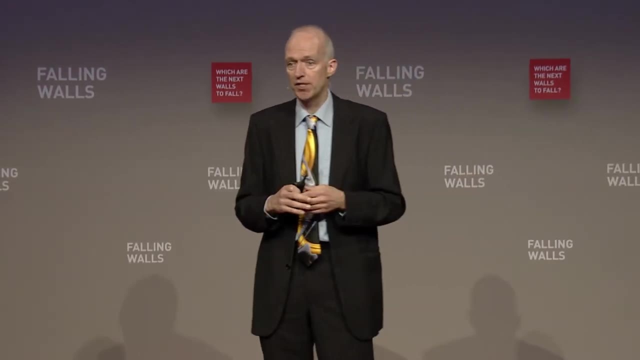 years of discussions. John Kerry was there, the Secretary of State at the time- and Obama really wanted an agreement on this. He wanted to have an agreement that we would not continue to use the HFCs in air-conditioning and refrigeration. 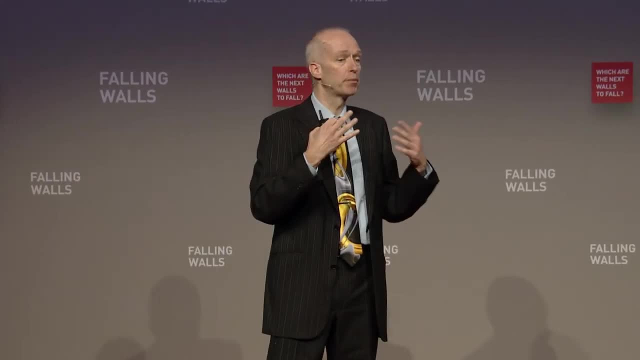 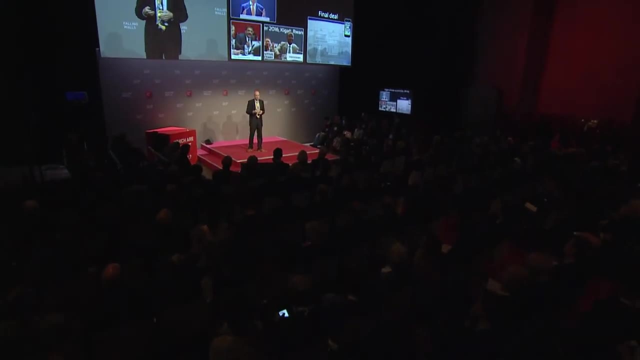 And they used an agreement, not the climate agreement- for it. they used the Montreux Protocol Agreement for it, because Montreux Protocol in fact caused the increase of HFCs, but they were the result of it And they made a final deal there. 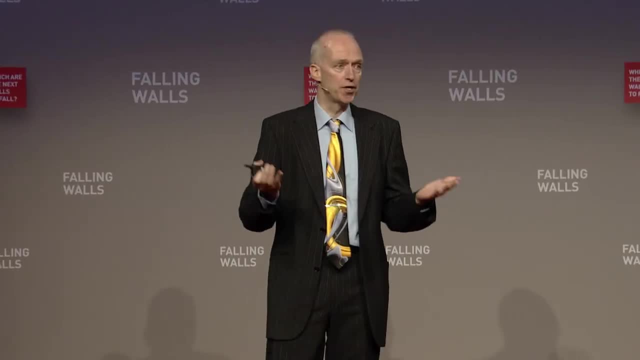 In the late hours of the discussions. they came up with a schedule there which shows a reduction. However, we're in the globe. We have to stop using HFCs. We have to stop using HFCs in the coming two or three decades. 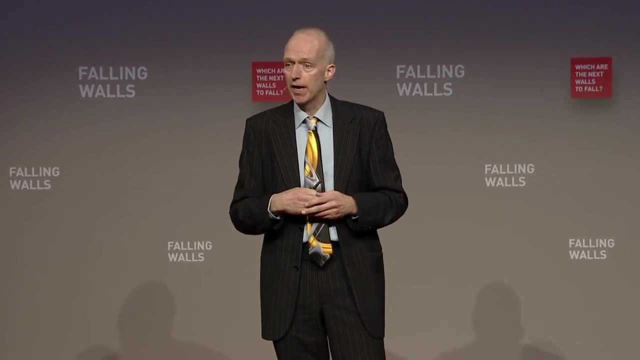 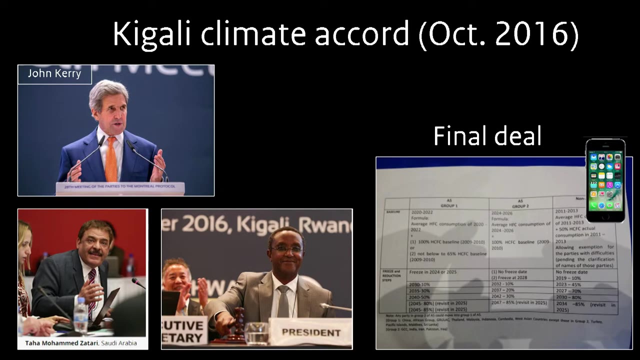 And I was present there, I made with my iPhone, I made a picture of the schedule and I thought, hey, I can calculate this. Just at the side, there, during discussions, when they were drafting the legal text, I calculated the climate effect of this agreement and communicated with the policymakers. 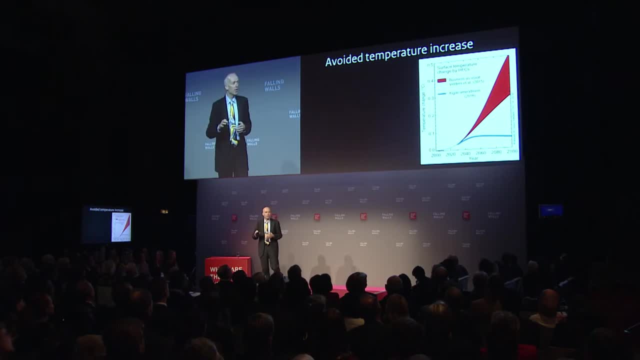 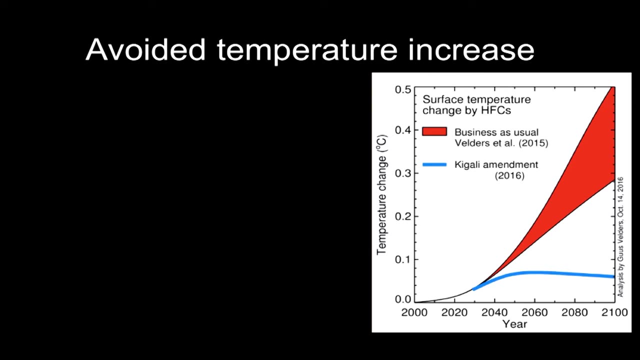 What I calculated was that. you see the red curve. that's without any agreement. the HFCs could contribute by the end of the century up to half a degree of extra warming of the surface. That's reduced to about .06 degrees Celsius, so a reduction of three to four-tenths of a. 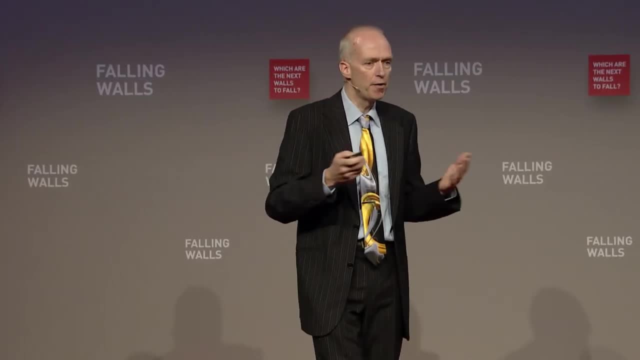 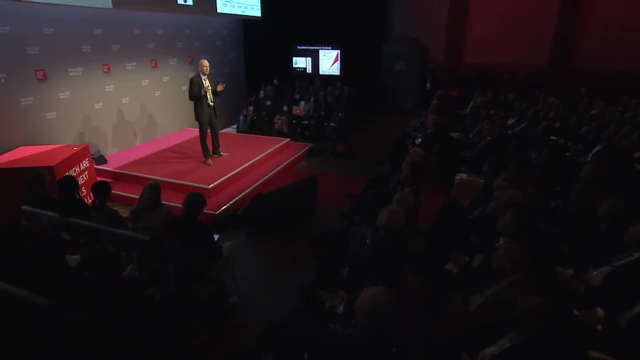 degree Celsius. And then you have to think. if you think maybe not a big deal, then you have to think about the Paris Agreement. They're not talking about it and two years ago they decided you have to limit the warming to one and a half to two degrees Celsius. 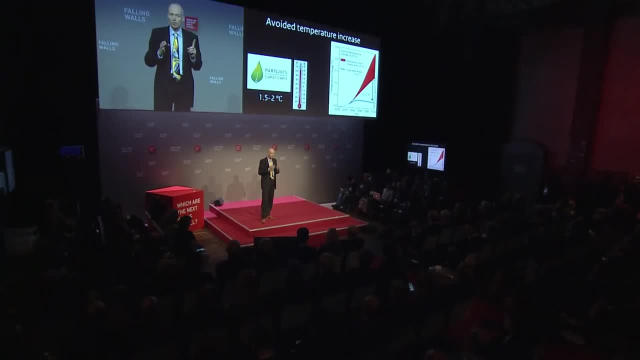 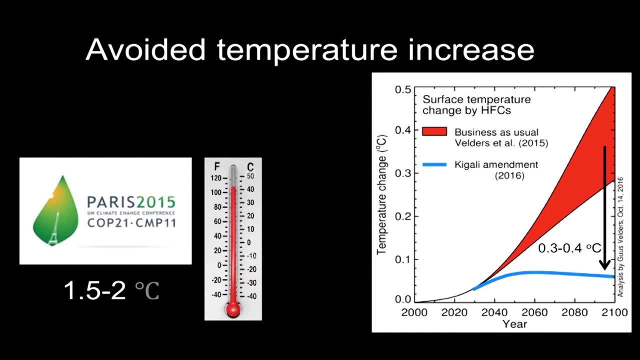 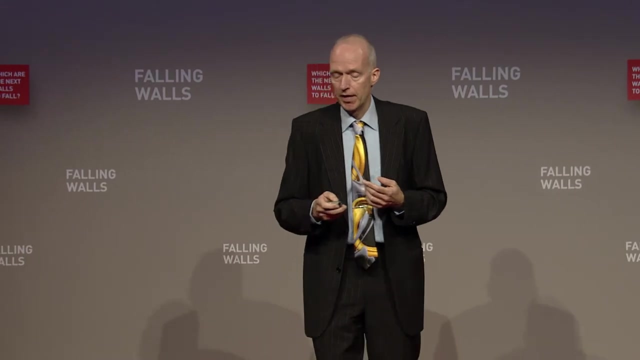 And of that one and a half or two degrees, one degree is already attained. We cannot do anything about the one degree. So we have only one degree to go if we want to stay below the two degrees Celsius, And then a few tenths of a degree Celsius reduction there is quite significant. 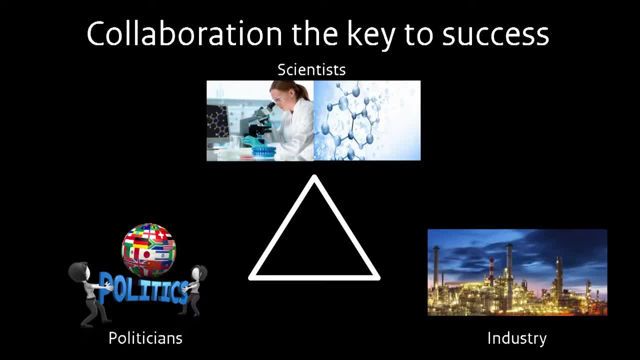 What I think was the key to success here. that was that scientists- they lead the way for the policymakers and industry to give them the signals, what's happening in the world. And in this case I could take up that role, But also industry was very active. 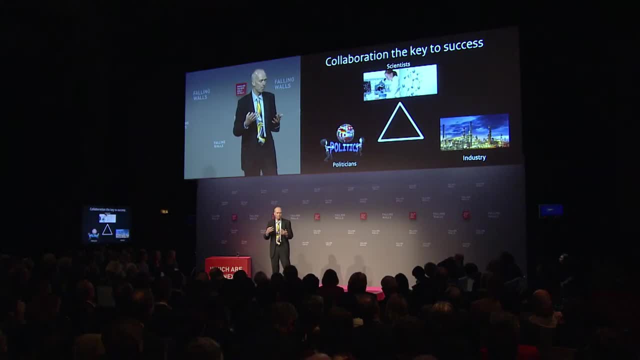 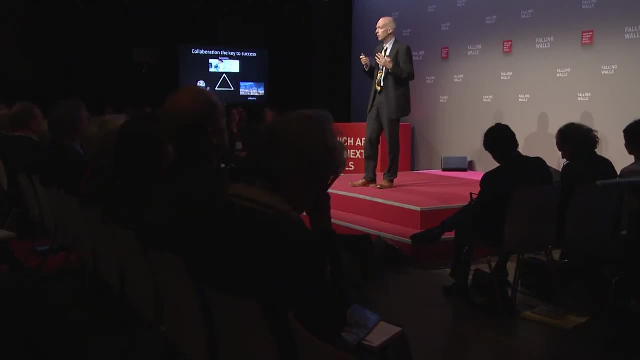 You want to participate, you want to invent new solutions to this problem. so they were on board And also politicians were very active here. Not only that, Not all the politicians from the beginning, but there was a good consensus in the whole community that action should be committed here. 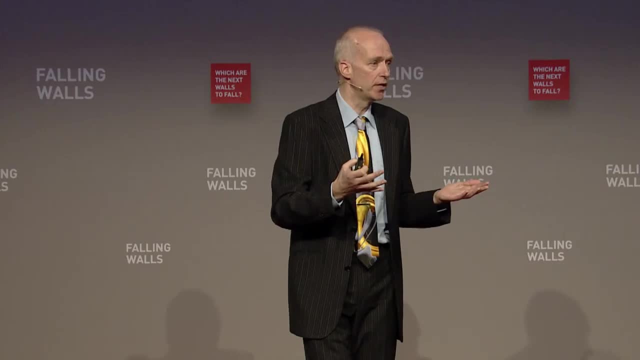 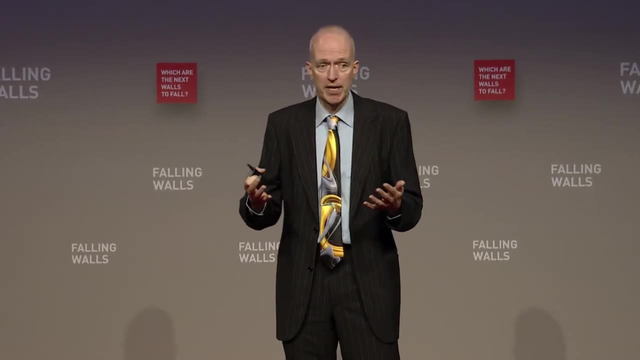 But of course it all comes down to the people, The people sitting in the room there, and not only the politicians, the industry people and the scientists, but also the NGOs who were there and the press people were there. They were all on board on this and there were no adversaries. 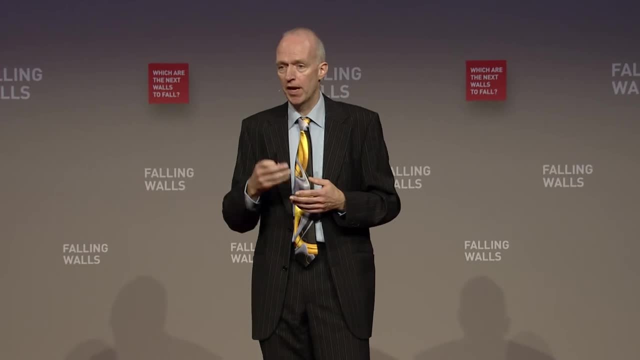 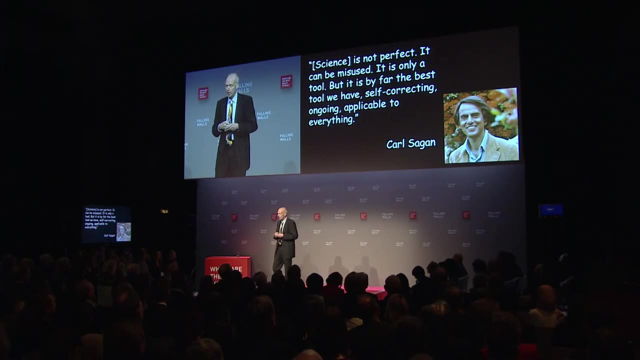 Everybody respected each other's position, but they all wanted to make steps forward. I think that was a big key to success. I go back to Carl Sagan. What he wrote, that science is not perfect, he said, and it can be misused.